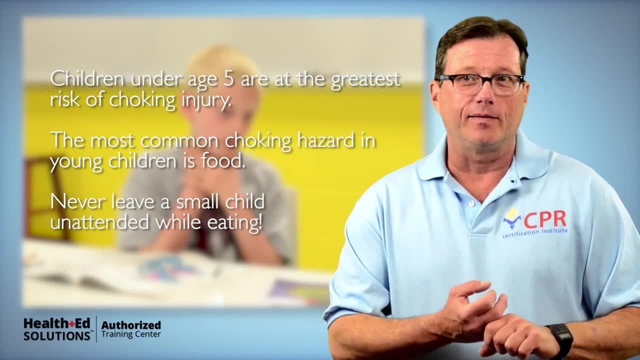 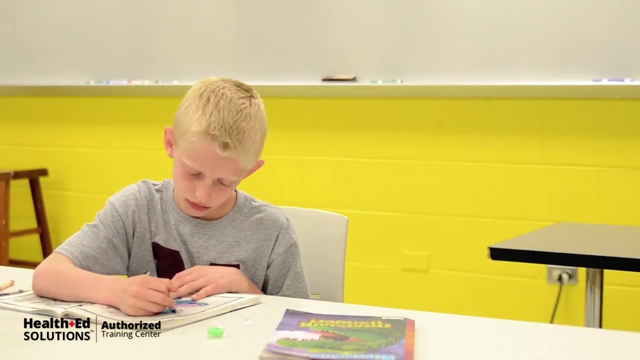 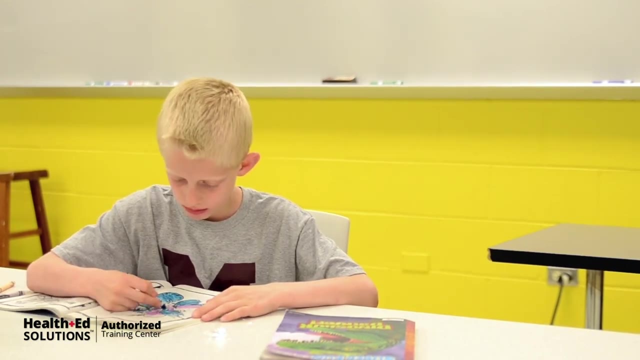 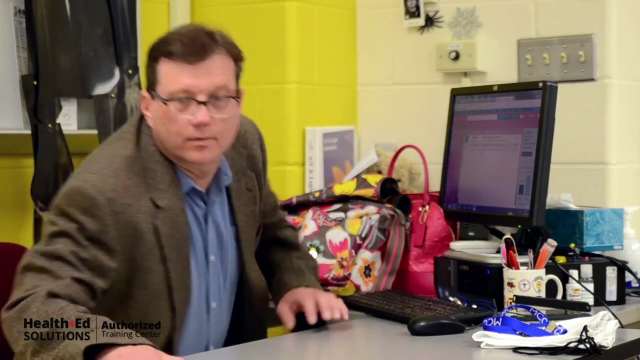 prevent that. Don't rush your child when they're eating and don't leave them eating unattended. Stay with your kid if they're eating, especially if they're under age five. First, recognize the choking victim. Recognize the child is choking. 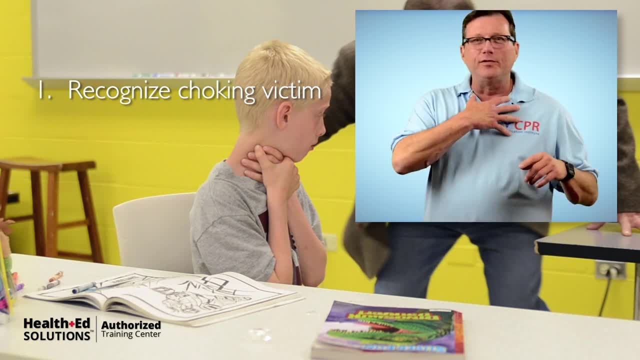 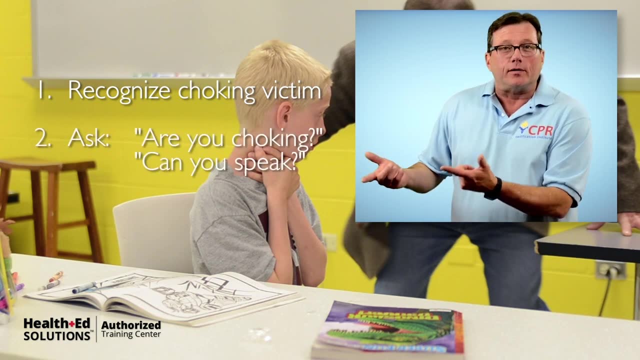 They might not be able to speak. They're going to look scared. They may be gesturing toward their throat. The only sound you hear coming out of them is a high-pitched whistle. Ask them: are you choking, Can you speak? If not, begin the Heimlich maneuver. Are you choking, Can you speak? 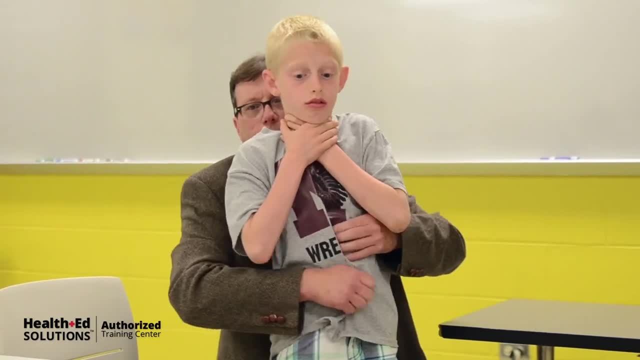 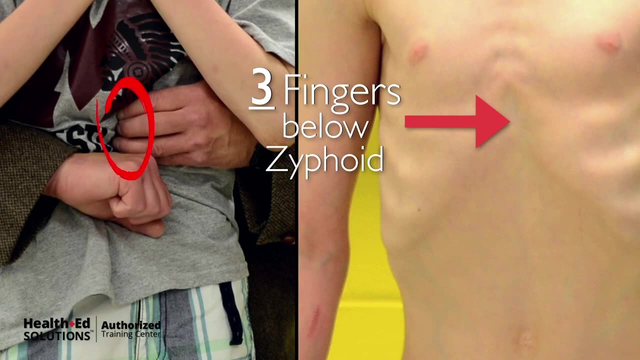 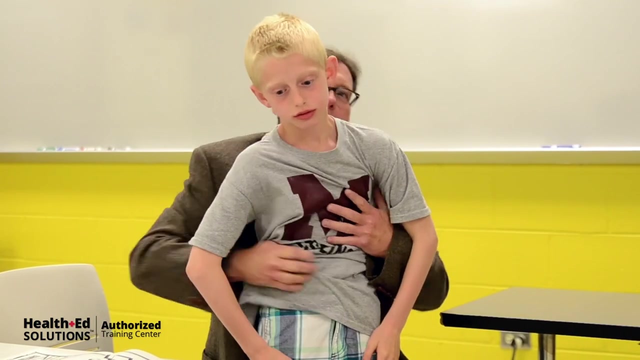 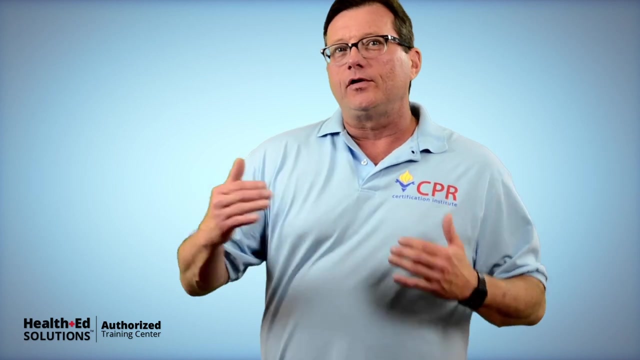 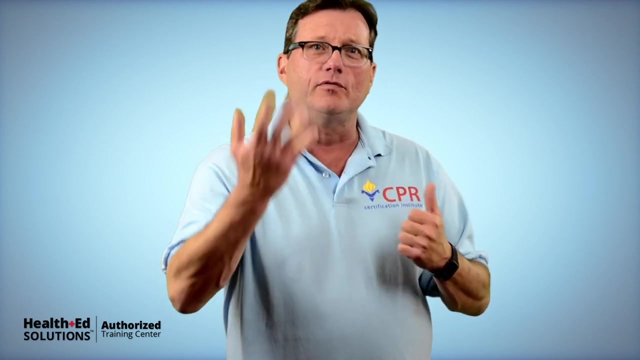 at all. Stand up. Now notice when you learned how to do the Heimlich on an adult. it was done standing. You're trying to get your hands underneath the diaphragm. You want to push up on the diaphragm to remove that object, but you can't do it hovering over. You have to get down. 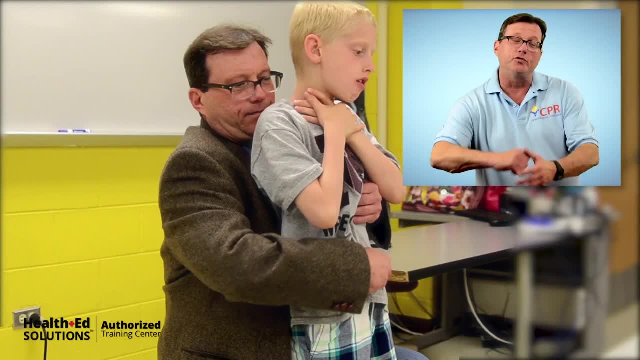 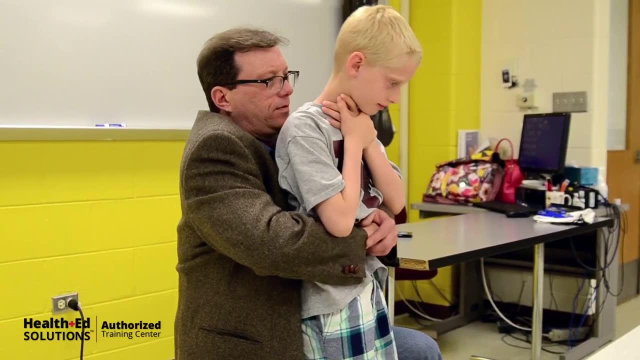 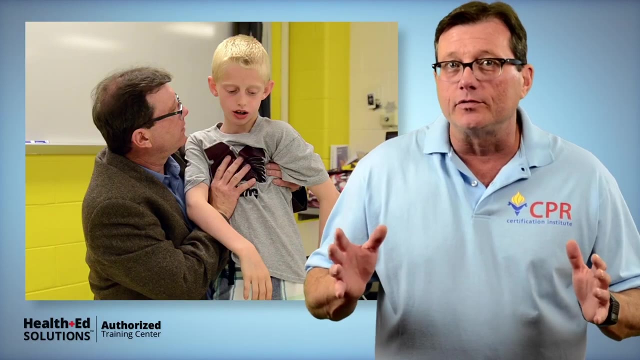 behind them. So drop down to one knee behind the victim. It puts you in a better position to do Proper effective abdominal thrusts. Now, after the object's been expelled, stay with the child, Make sure the child is okay. 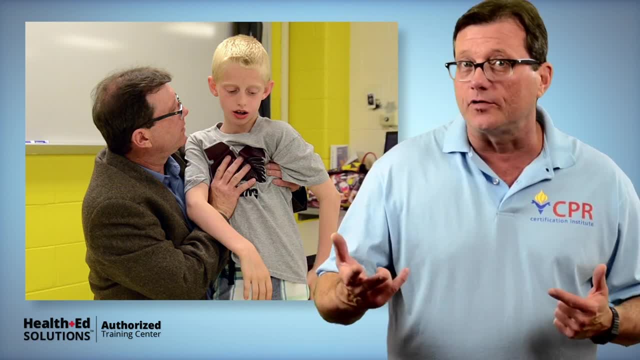 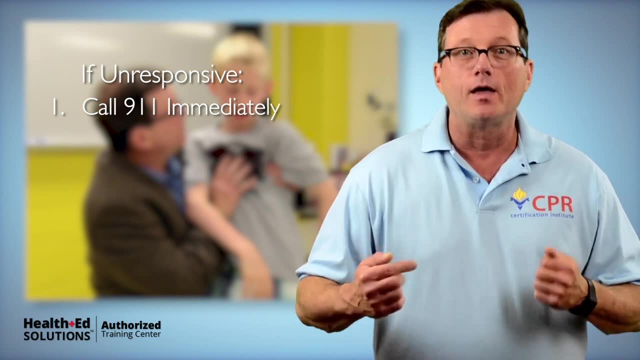 You're going to continue to do the Heimlich maneuver until either the obstruction comes up or the child becomes unresponsive. At this point, call 911 immediately. Get some help coming, Come back, Begin CPR. You're going to start standard CPR. 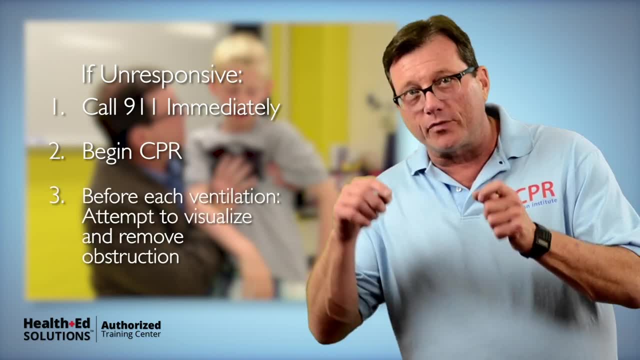 There aren't too many differences. Before you put air into the victim, open up the mouth, look in the mouth, see if you can visualize the obstruction and pull it out.